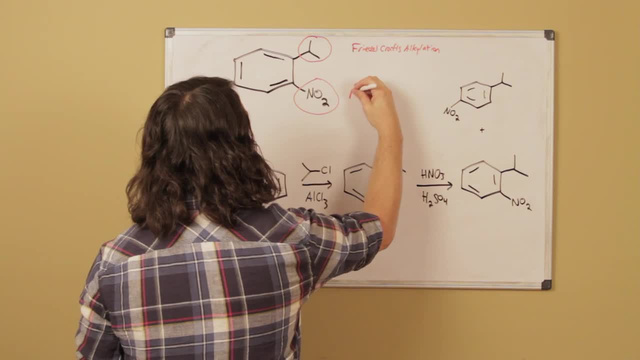 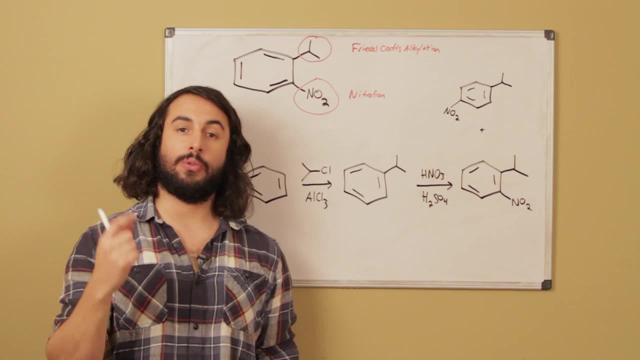 ok, and then we also have a nitro group and we know that a nitro group can be attached to a benzene ring by nitration. so we know that we're going to do a Friedel-Crafts alkylation and we know that we're going to do a nitration. but what order are we? 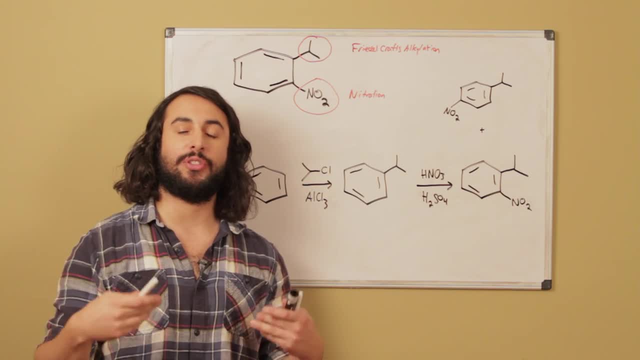 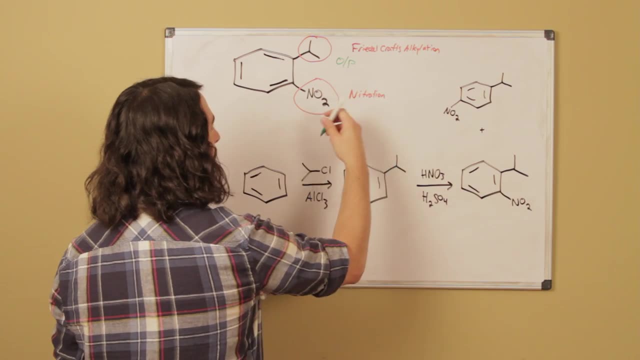 going to do them in? in order to answer this question, we have to understand something about the directing abilities of these groups. now we know that an alkyl group is an ortho-para director, and we know that a nitro group is a meta director, and we also understand that the 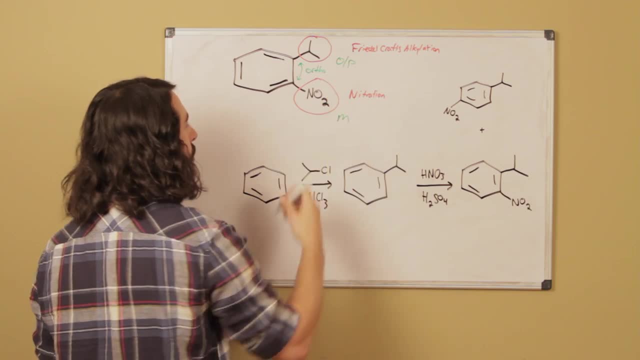 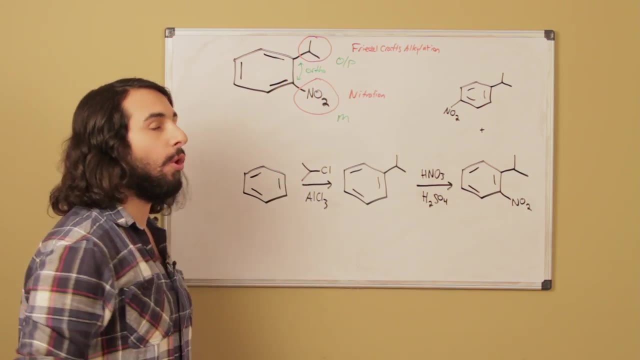 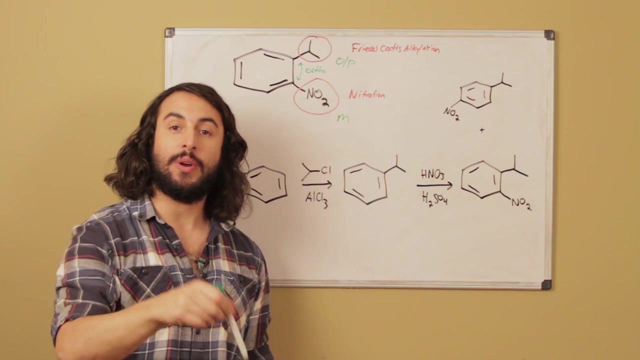 relationship between them on the molecule is ortho. so this is going to tell us what order we have to do the reactions in, because, given that they have an ortho relationship to one another, it must be the ortho-para director that directed the other group to its position. and so what we're saying? 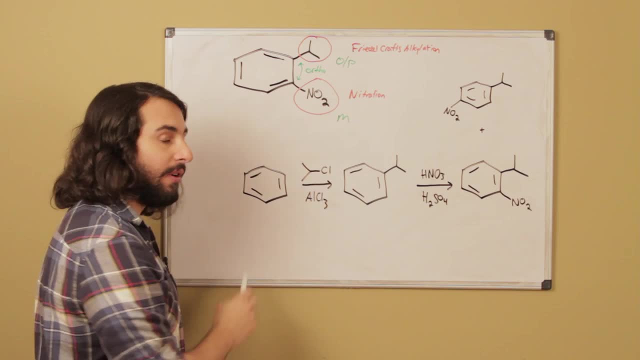 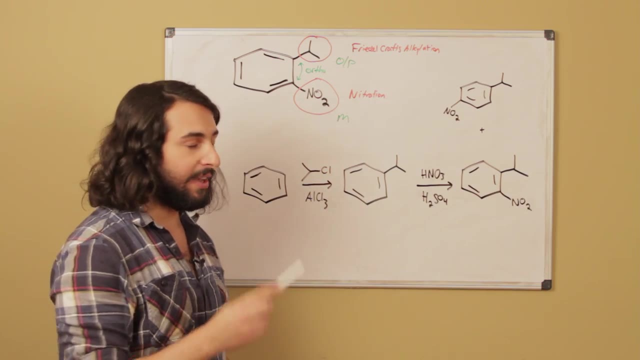 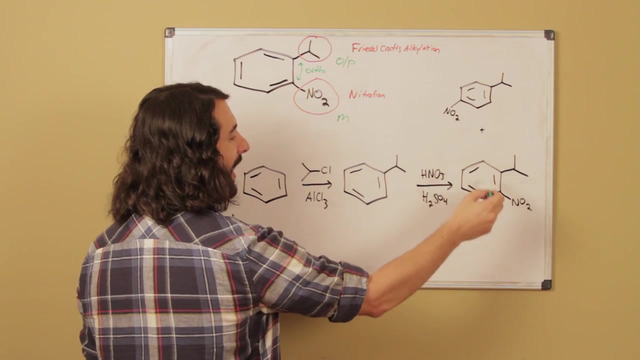 is that we must, starting with benzene, have done the Friedel-Crafts alkylation here with this alkyl chloride to get this intermediate. because if we have this intermediate then upon nitration we will get a mixture of ortho and para nitrated products, whereas if we were to do the 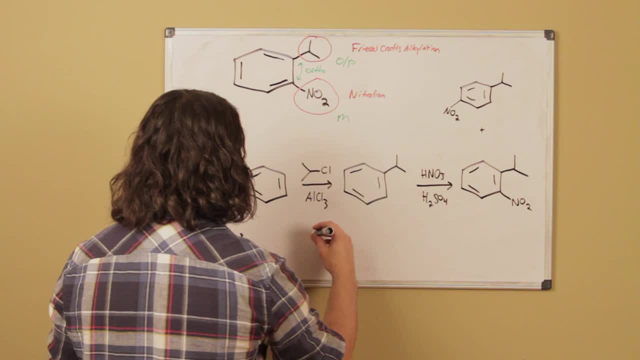 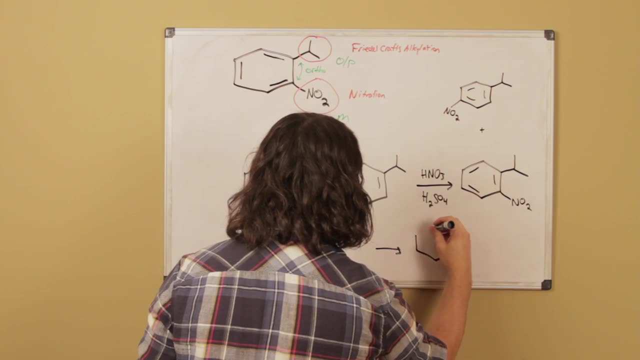 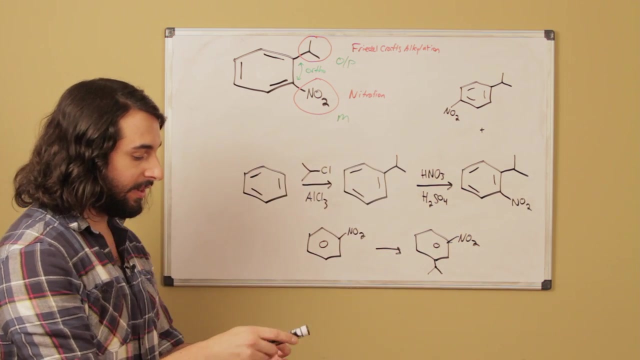 nitration first. if we did the nitration first- and let's say this was our nitrated product- then if we went and did the alkylation, we would get meta direction from the nitro group, and so the nitro group cannot have this have been the compound that was added. 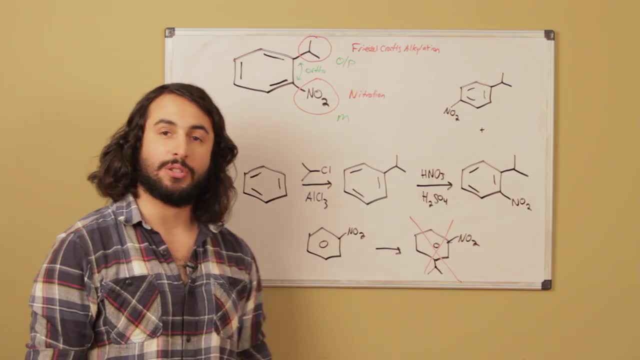 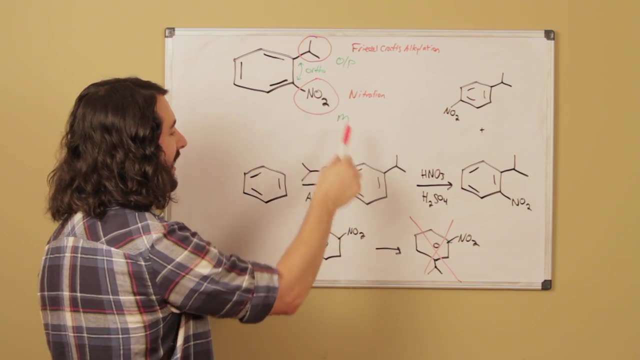 first, because that will not give us a structure that matches our target molecule. instead, we're recognizing that alkyl is orthopara, nitro group is meta, so it must have been the alkyl group that directed the nitro group to the ortho position. we can get this mixture. 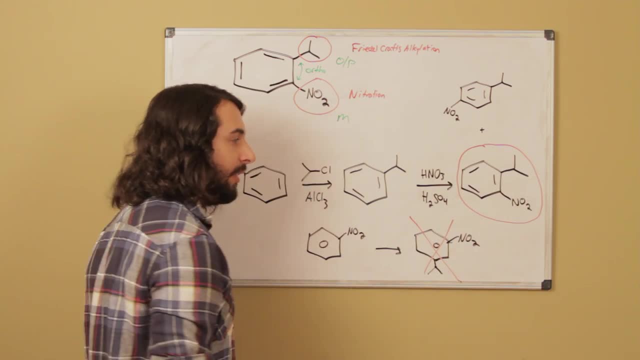 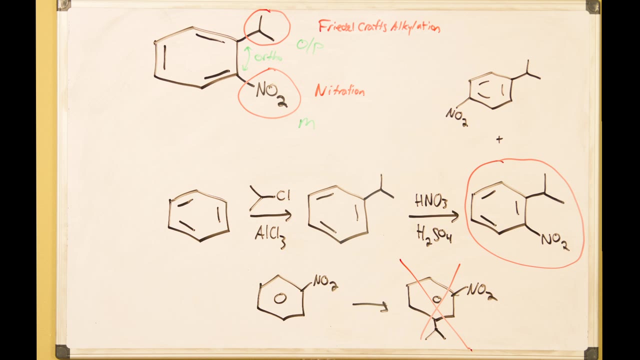 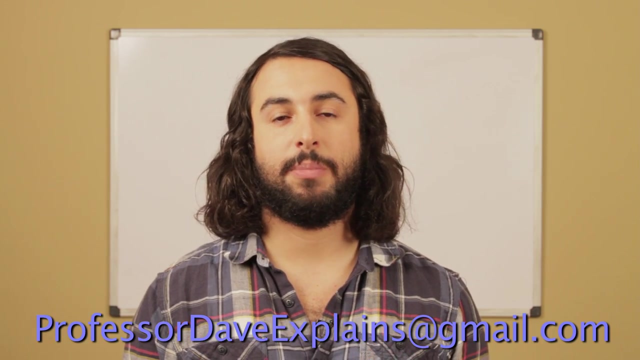 separate them out and there is going to be our target molecule. Thanks for watching, guys. subscribe to my channel for more tutorials and, as always, feel free to email me professordaveexplains at gmailcom.